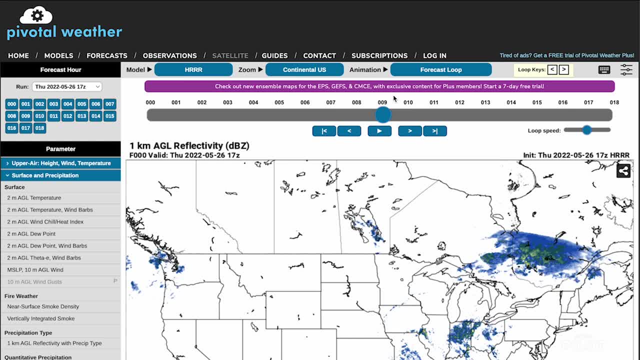 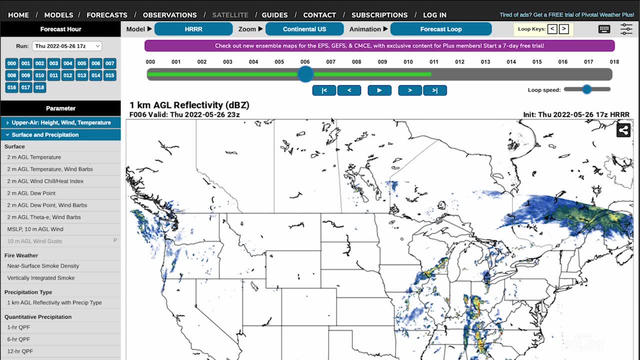 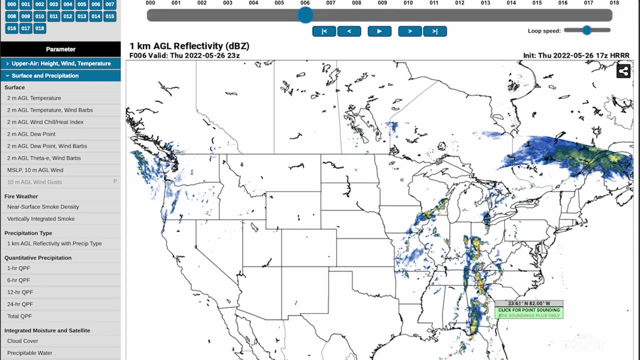 where it says single image, select forecast loop: okay, and now you see it's building the image for us. Okay, so we can see right off the bat that there's something going on in the southeast. okay, So what we'll do is we'll just animate it, okay, And then you 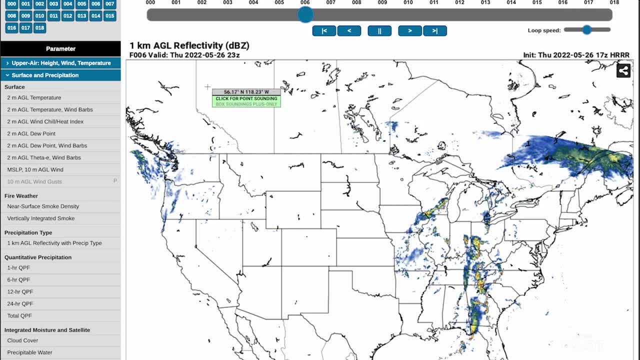 can see that 11 Zulu it goes up to 11 Zulu. It goes 7,, 8,, 9,, 10,, 11,, 12,, 13,, 14,, 15,, 16,, 17,, 18,, 19,, 20,, 21,, 22,, 23,, 24,, 25,, 26,, 27,, 28,, 29,, 30,, 31,, 32,, 33,, 34,, 35,, 36,, 37,, 38,, 38,, 38,. 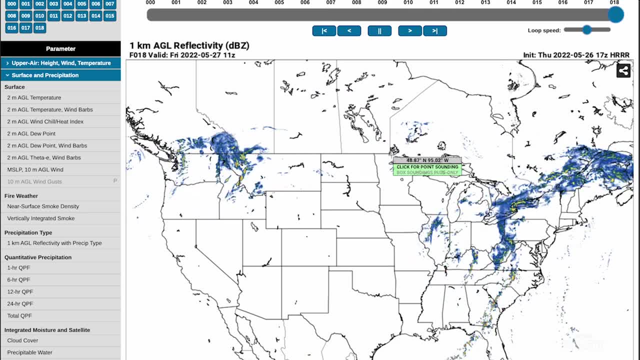 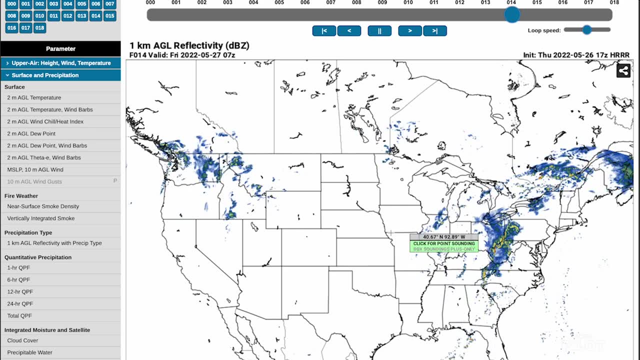 39, 40. It goes 7,, 8,, 9,, 10 hours into the future, which can be very helpful. You see, there's something happening here. There's a rotation here That's the parent, low and 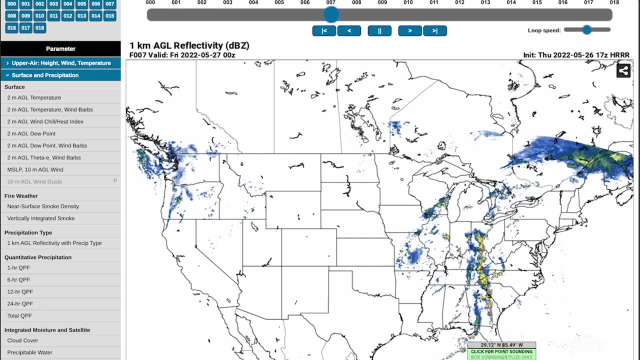 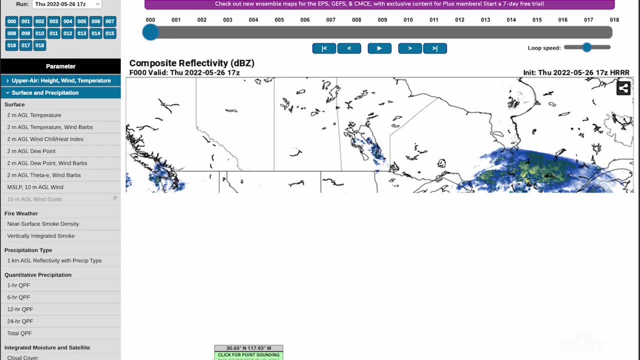 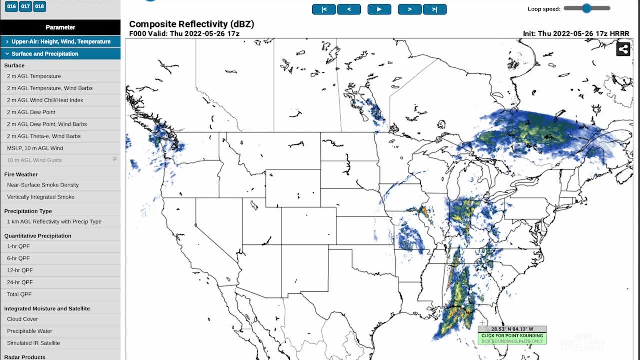 this is the front going up and down in the north. there It looks like some of the strongest echoes down there. We can also select composite reflectivity, which is the totality of all the returns on the on the radar screen that the model is prepared And you can see that it's a lot. 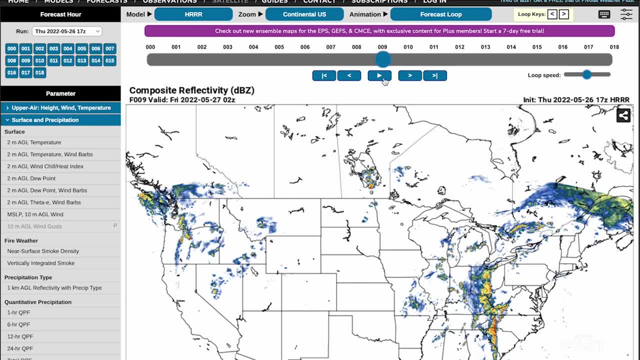 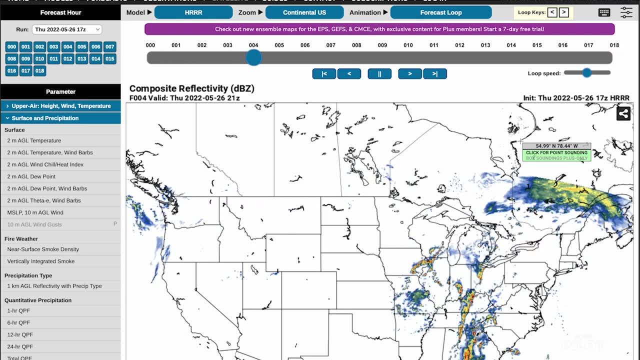 heavier precip because it's sampling the entire air column So we can animate that and see how that's going. So you know that if you're going to be departing in three hours, this gives you a pretty good idea of what you can expect. 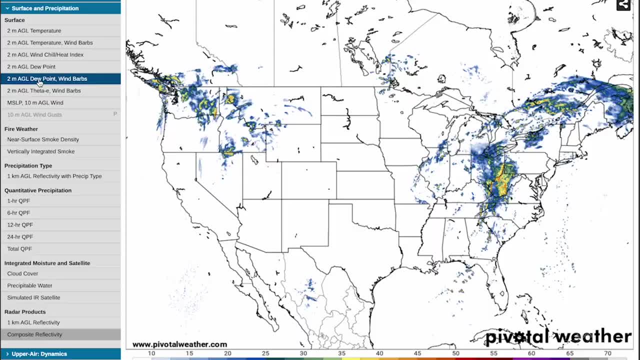 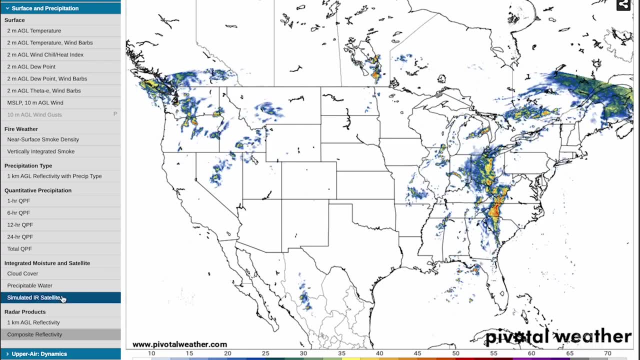 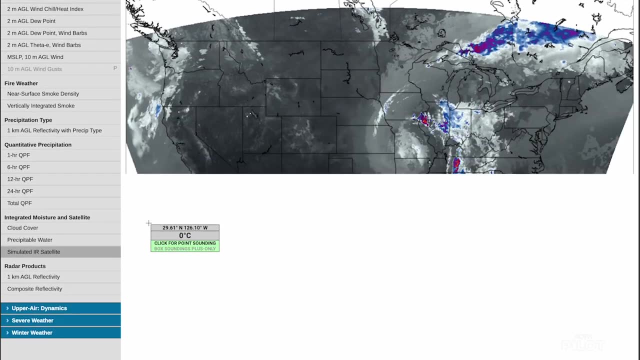 Some of the other products you can select from this whole list here is very, very interesting. It's interesting for sampling a number of other products. It makes a simulated infrared image, So this is like if you're looking at a satellite image of it. Here you see this. 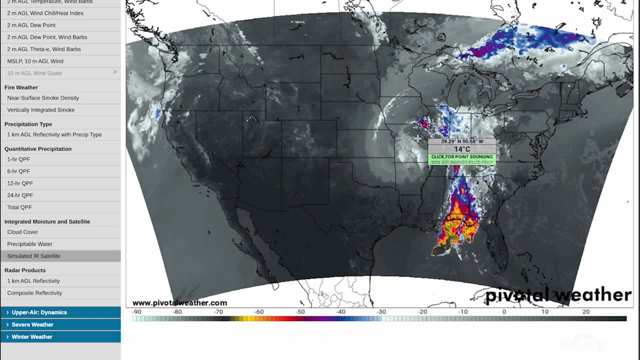 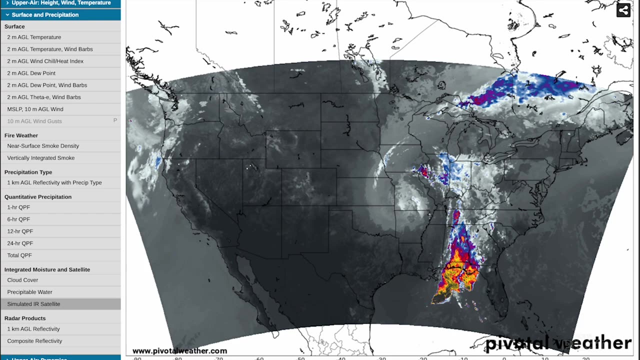 circulation because it has clouds and precip. This is the circulation around the low in Missouri right now and you can see this huge fetch of moisture and storms coming off the Gulf into the panhandle of Florida And again go up here and you can animate it And we. 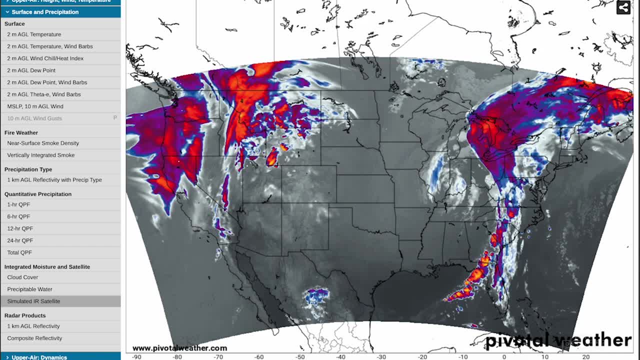 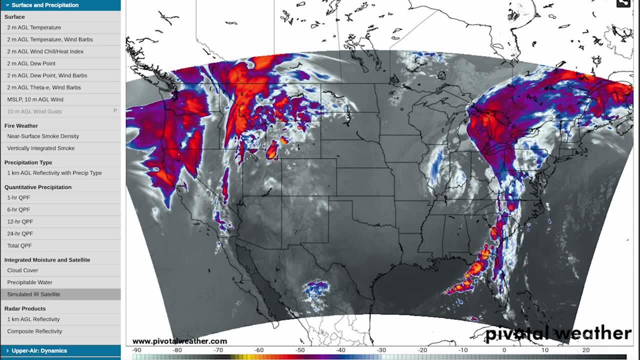 got a big system coming in off the West Coast So you can see now this, all this red and purple. those are cloud tops. So we know we saw that the rain was kind of skimpy, except down around the panhandle of Florida, But look, you got huge cloud tops and this means 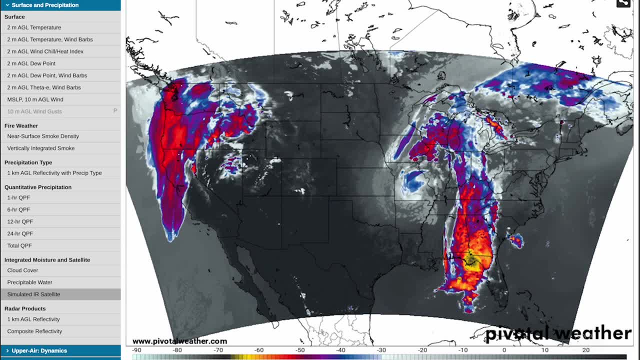 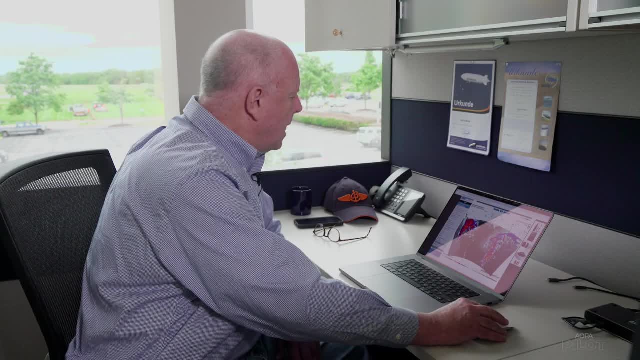 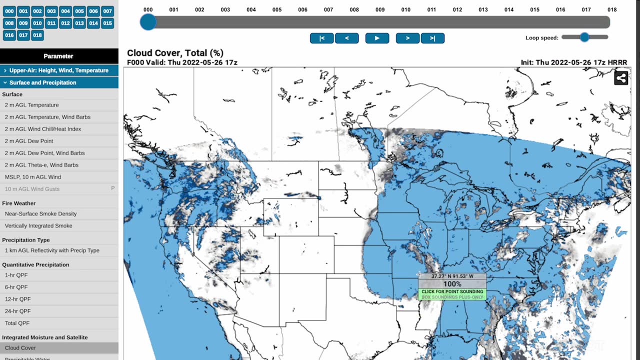 big trouble because the red, purple shades Show cloud tops up in the 40,000-foot range: 35,, 40,, 45.. Another cool thing: cloud cover. Click on that. So this whole comma-shaped image here, that's your low-pressure center. 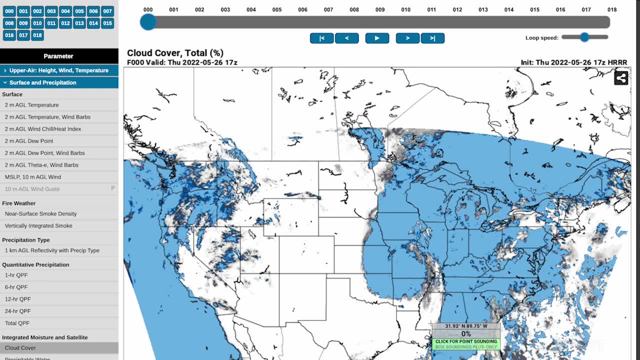 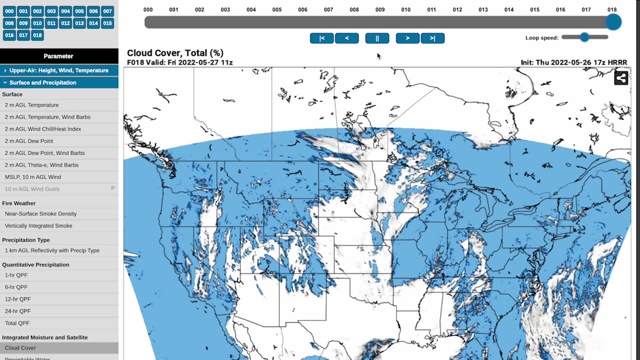 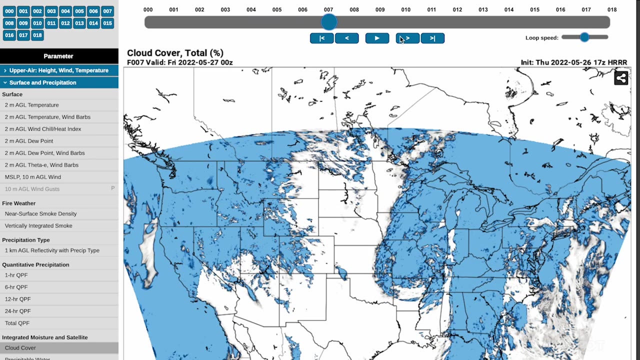 and this is the front. You can see the cloud's very sharp line there and that's the front. all right, I mean, there's nothing subtle about this thing. There's a cold front coming And again you can animate it or you can go hour by hour to see where clear spots might be. I 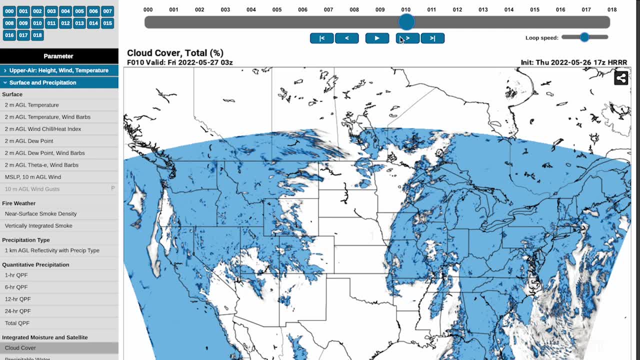 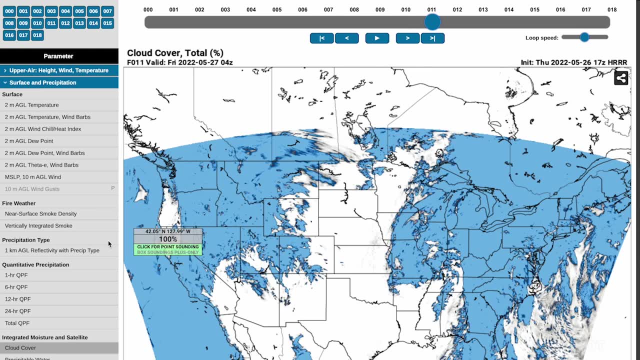 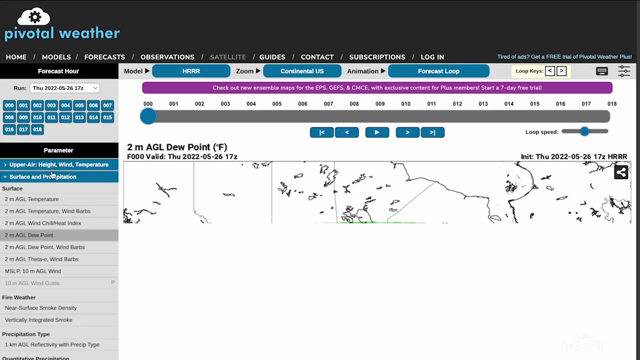 don't think I'd bet on any of this, But again, because it comes out every hour, it's much more accurate because it's more timely, Its sampling rate is higher. Some other things you can look at: dew point is interesting to look at because this helps. 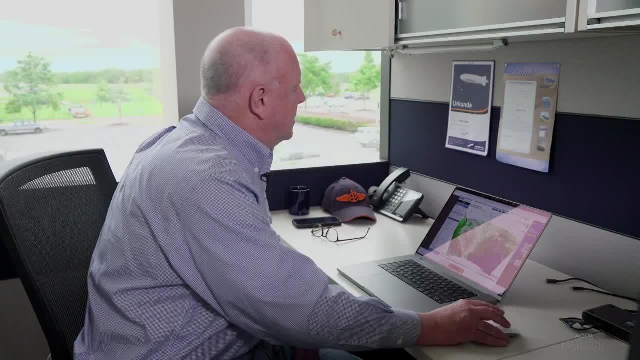 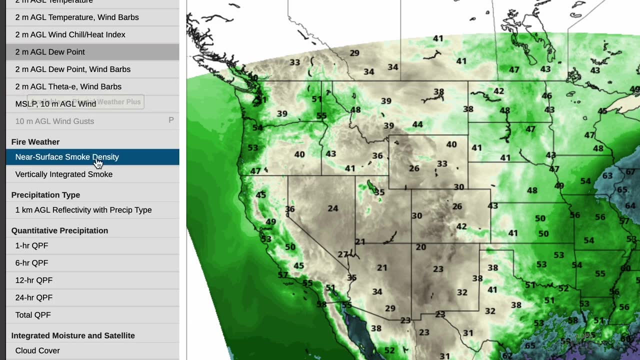 you identify the front even more And you can show some other things. It has a bar here for wind chill for winter time. The closest thing that you would have to something like what we've been looking at is the wind. I'm going to go ahead and show you some of the things that we've been looking at And 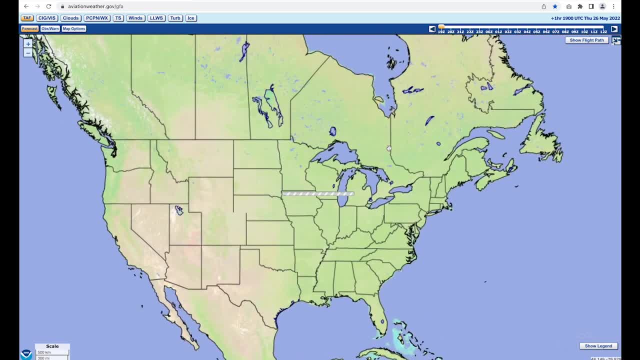 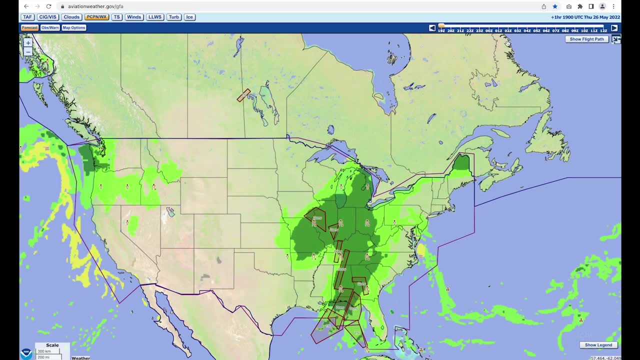 I'm going to show you some of the things that we've been looking at And I'm going to show you a graphical forecast for aviation tool where you can pick precipitation- It's not initialized as often, as rapidly or as frequently as the HRRR is- And you can animate. 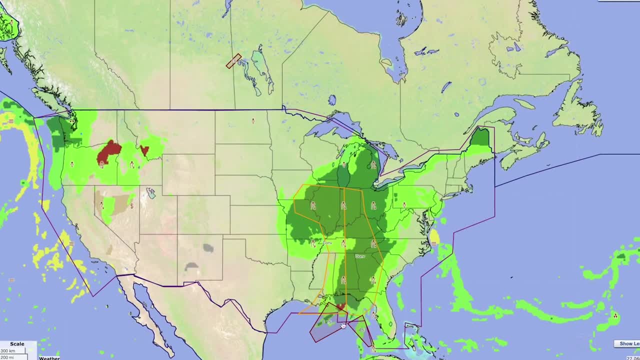 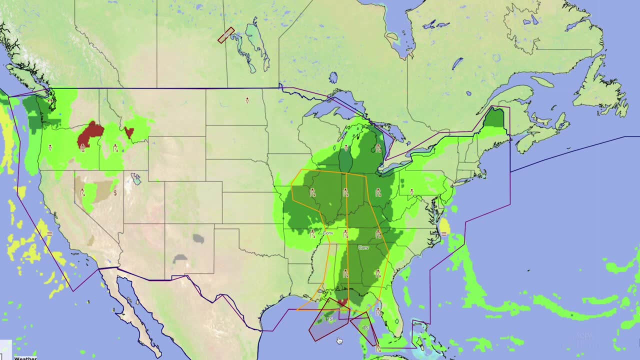 it as well. The advantage here is that it's actually putting the sigmets in here And we can see down in the gulf where we saw that headlight, We saw that heavy flow of moisture coming in off the gulf into the panhandle.